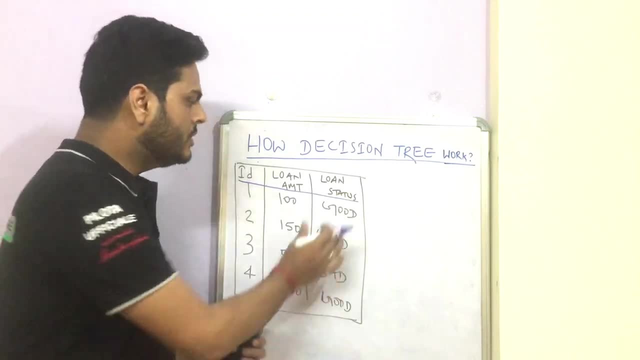 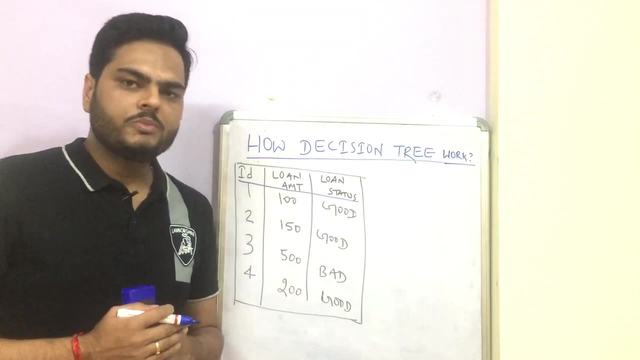 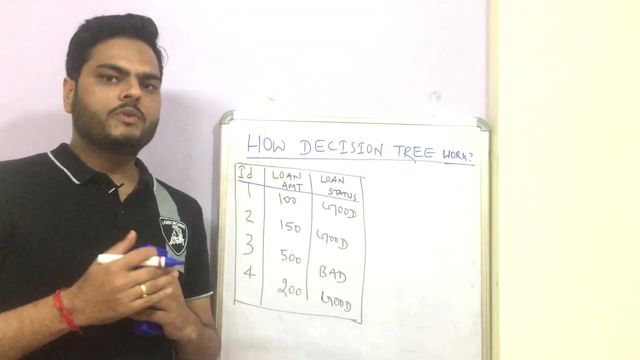 customer and whether that loan turned out to be a good loan or bad loan. Welcome to OneFold Data Science. My name is Aman and I am a data scientist. In this video, I am going to make decision trees absolutely clear for you using this simple data. Let's start So. first of all, what is decision tree? 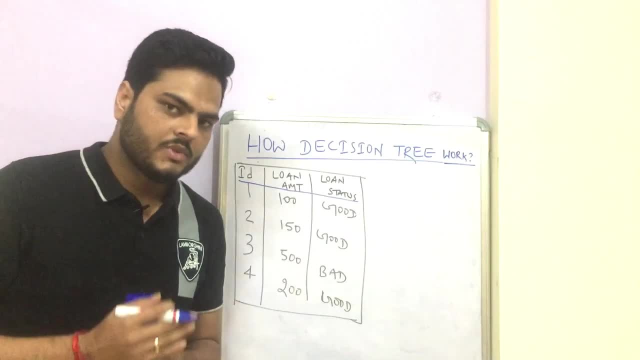 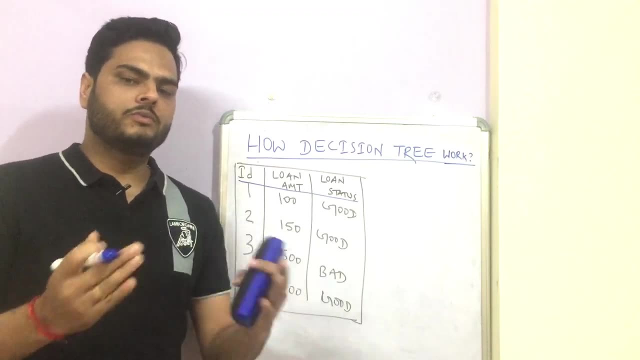 Decision tree is nothing but a machine learning algorithm. What is a machine learning algorithm? A machine learning algorithm is a way in which machine learns the pattern from the data. You can see this video coming as suggestion and you will be very clear on what is machine learning and what. 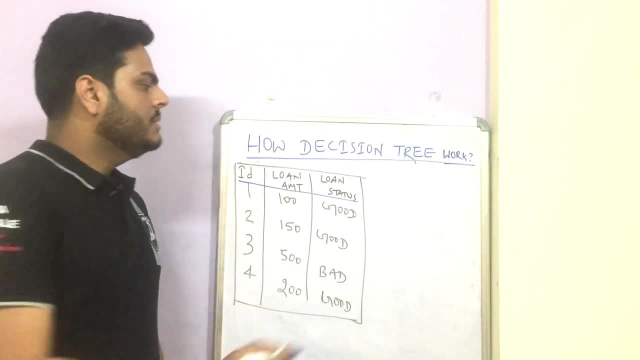 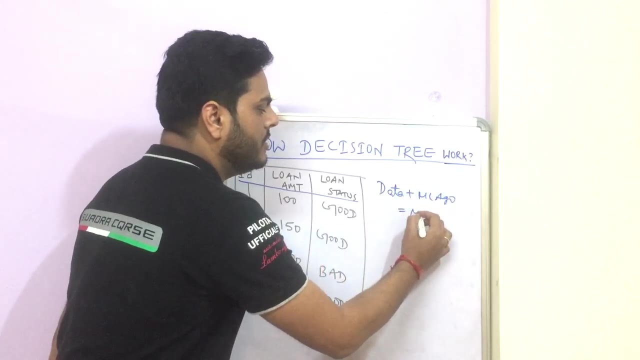 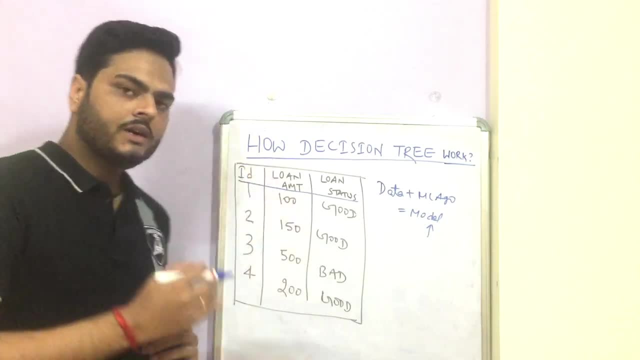 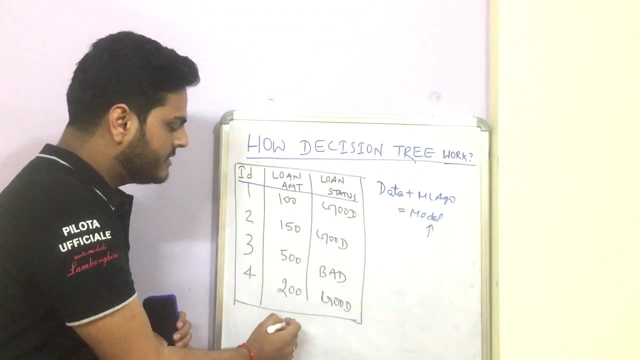 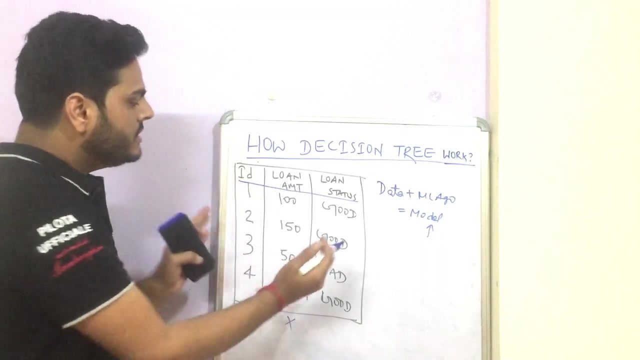 from the data. So if I create a model from this data, then tomorrow this model can answer my question. if I ask this model- hey, the loan amount is X- Could you tell me what would be, whether this loan would be a good loan or bad loan? So that is the use of this model. So what is decision tree? 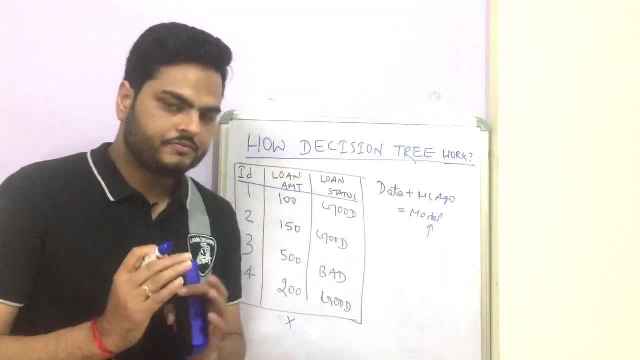 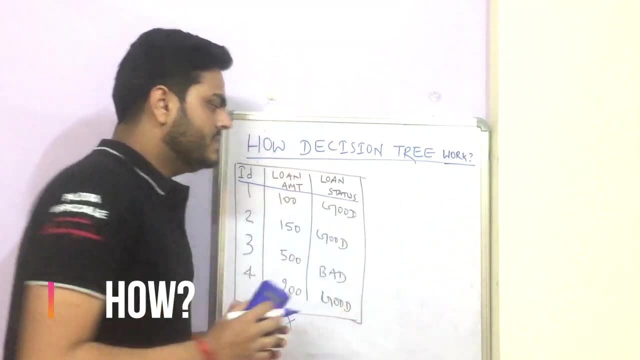 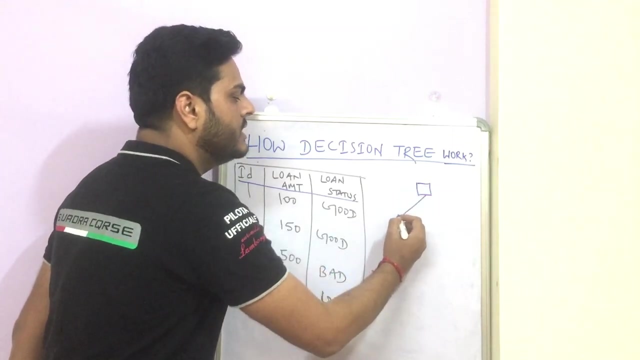 Decision tree is a way of learning the pattern. We will see how the pattern is learned in decision trees. So if we talk of decision tree, it typically works as a normal tree structure. So this is how a tree looks like: There are root and there are branches of the tree. So this is. 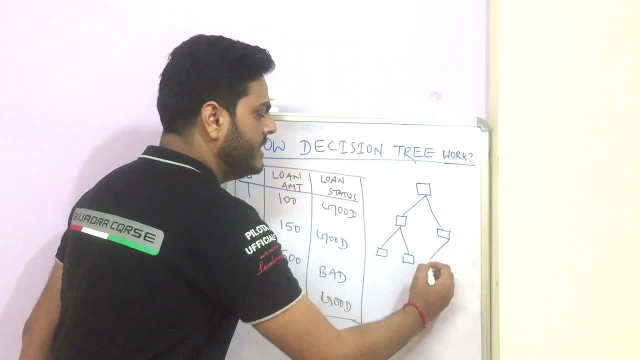 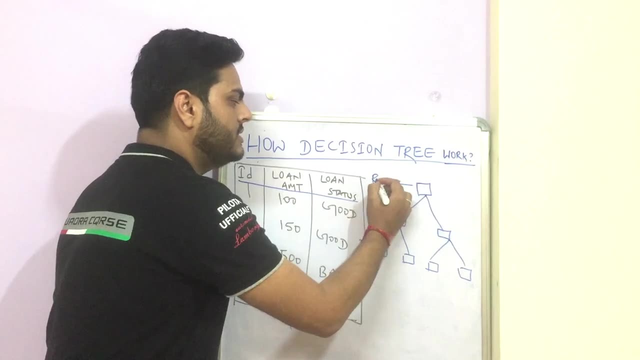 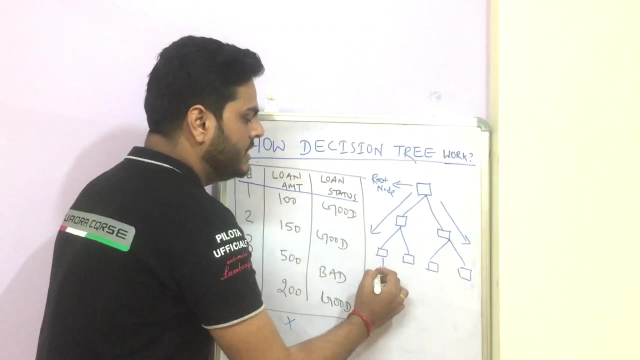 one branch and this is other branch and then it goes on. So this is how decision tree also works. So this is called root node in the language of decision trees, root node, and these are called different branches of the tree and these are called leaf. 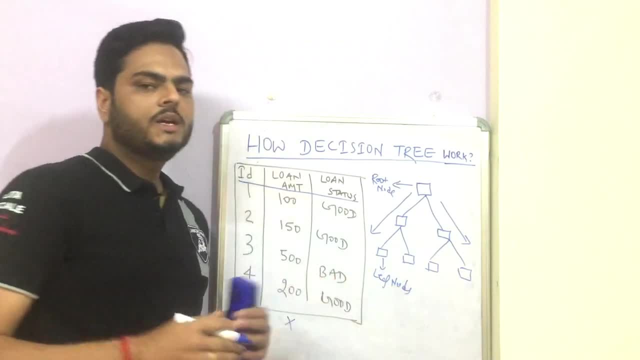 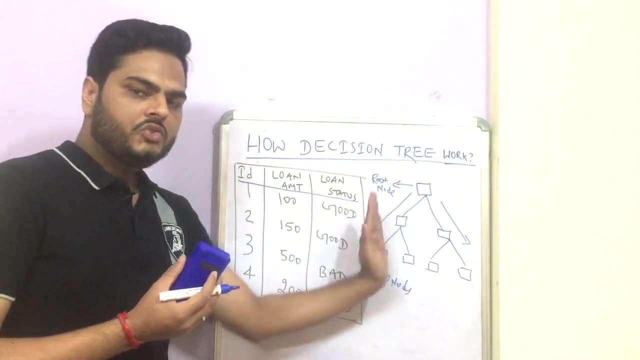 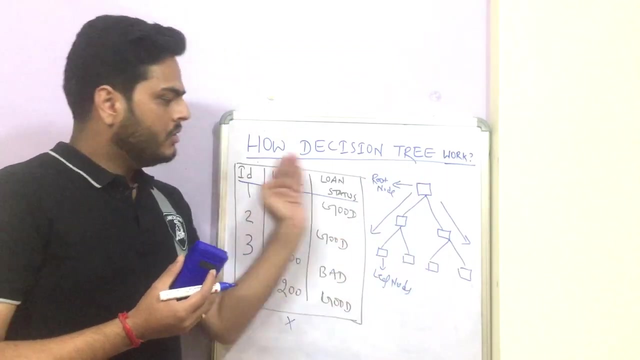 nodes. as these are the last nodes, So these are called leaf nodes. So these are the basic terminology of decision trees. Now how is this tree created? That tree is nothing but model. in this case, The tree is nothing but the pattern Which the algorithm has learned from the data. But how is this created? So let's say we take this: 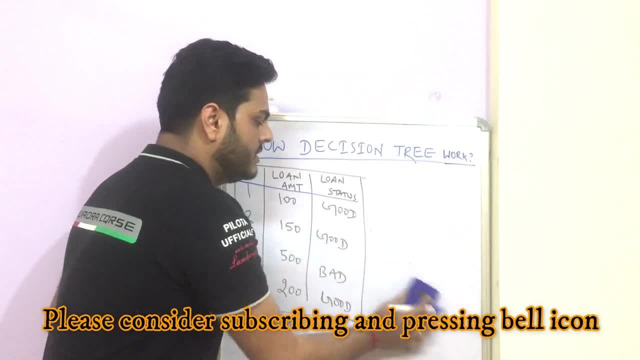 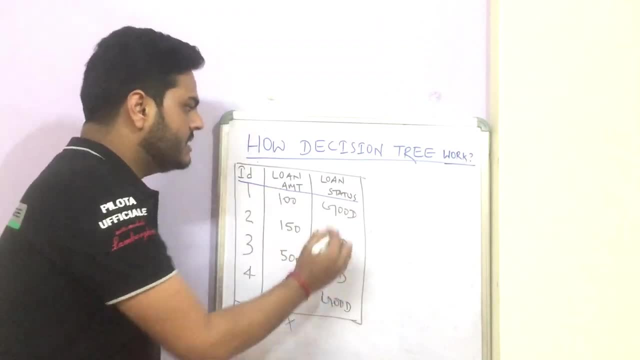 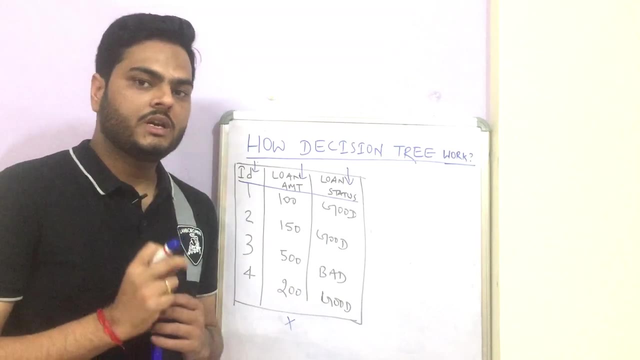 data and we submit this data to a decision tree algorithm. So what will happen here is: first of all, the root node gets selected. Now, in this example, this is the target column, and these two are independent variables of the data. All the independent variables are candidate for root. 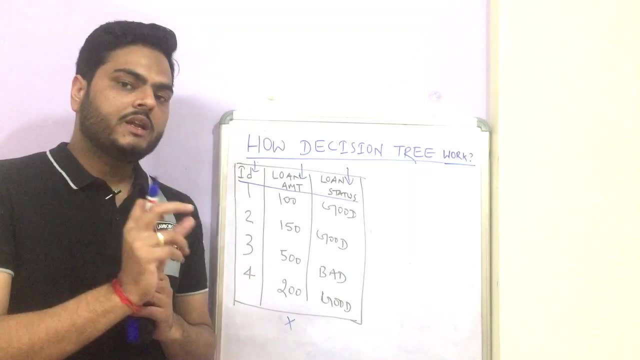 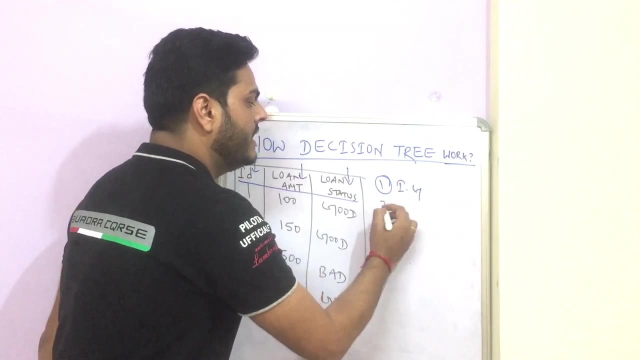 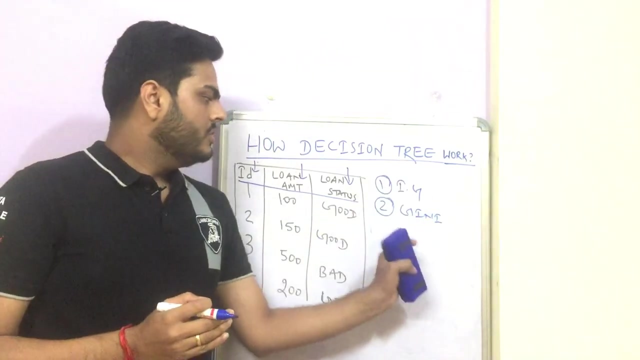 nodes, But which column will be selected As the root node depends on two criteria. One is called information gain, IG, and other is called Gini index, commonly known as Gini, or Gini people call it. So both these are the criteria on which 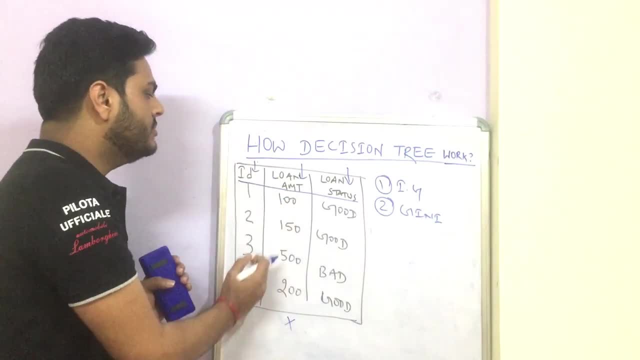 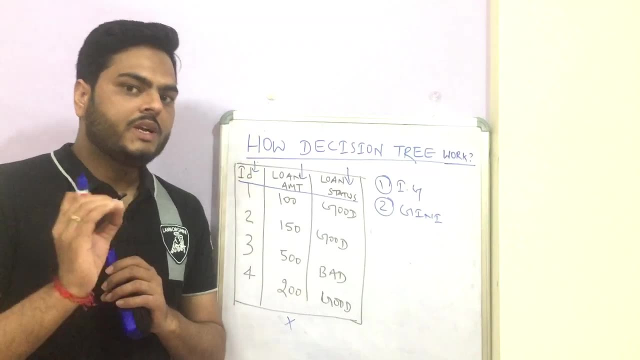 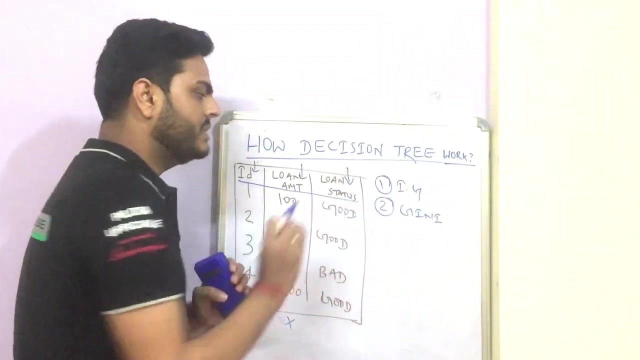 decision tree internally decides which column to select for the root node or subsequent nodes and what criteria to give as a filter. Okay, So these two things I'll separate. I'll create a separate video to explain these two topics, as these two topics are. 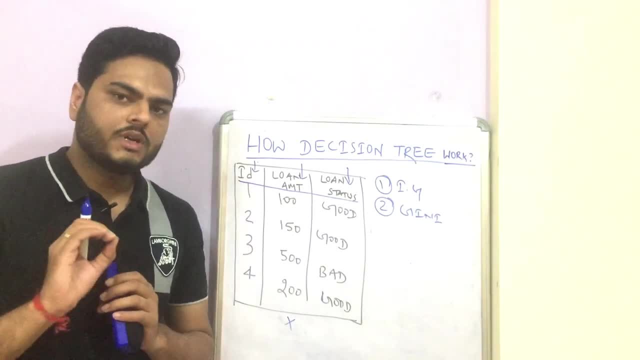 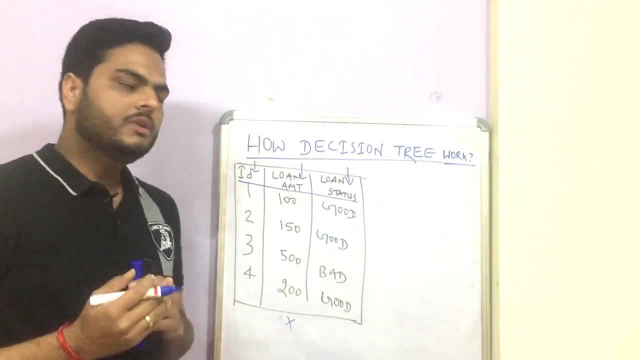 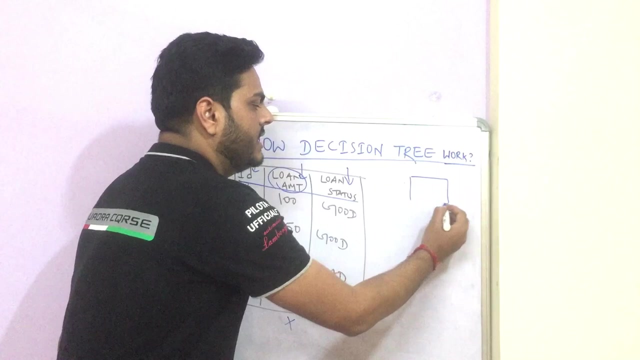 little mathematical in nature and very, very important topic. Okay, For now I'll give you a high level view of using these two: how decision trees created. So, let's say, this loan amount column gets selected using those criteria. Okay, So a root node will get created like this: loan amount. 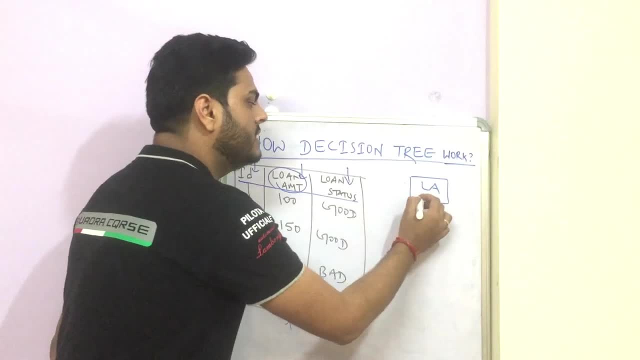 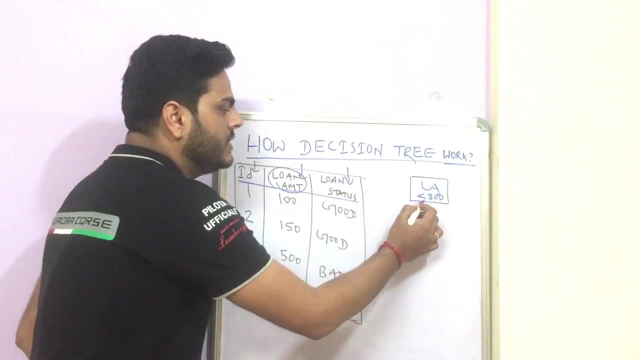 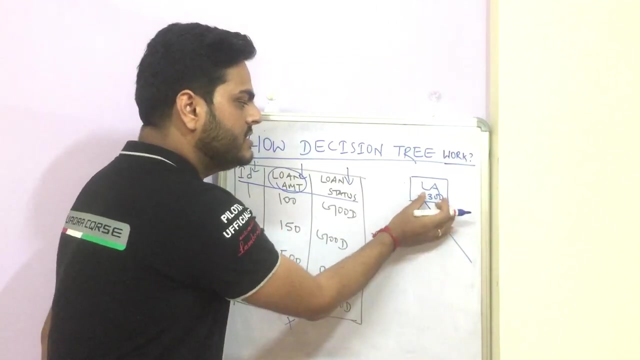 Okay, And then one condition. So let's say, loan amount greater than or less than three, And that is one condition, Okay. So loan amount less than 300, all the records will come from this side of the tree, which means one branch, and all the records, which is for where this, this condition is false, goes on other side of the branch. 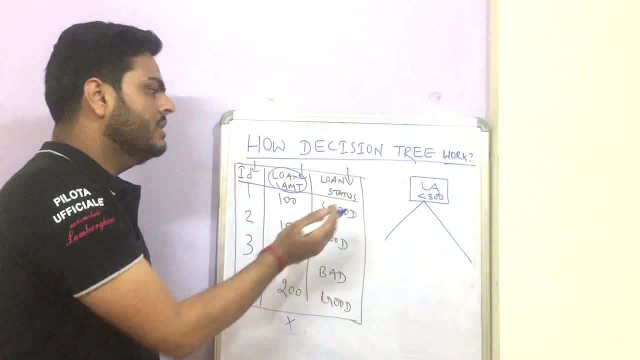 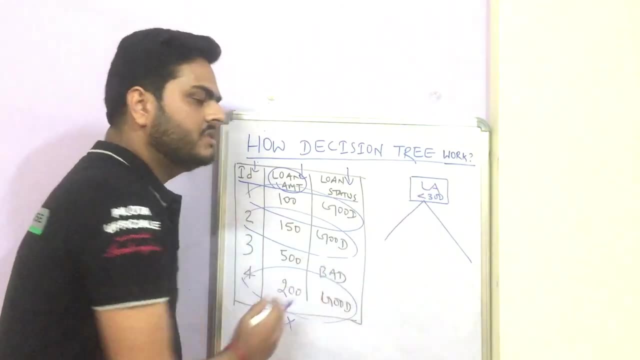 Okay, So how many records will come? this side of the tree, less than 300, this record, this record and this record: right, So this side of the tree, this side of the tree, in this branch, we will have three records. 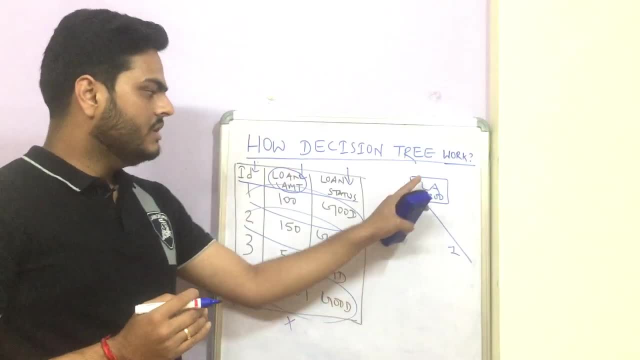 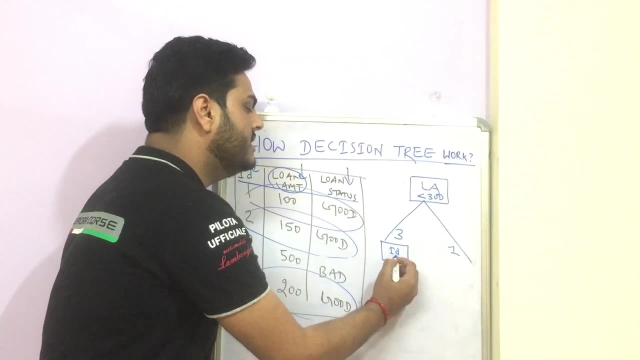 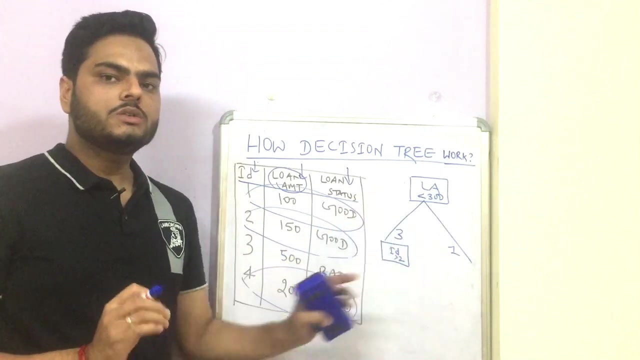 And here we will have one record. Okay, Further in these three records there can be one more branch of the tree for seeing ID, greater than two. again, which column to select and what criteria to select, depends on those two conditions only, mostly. 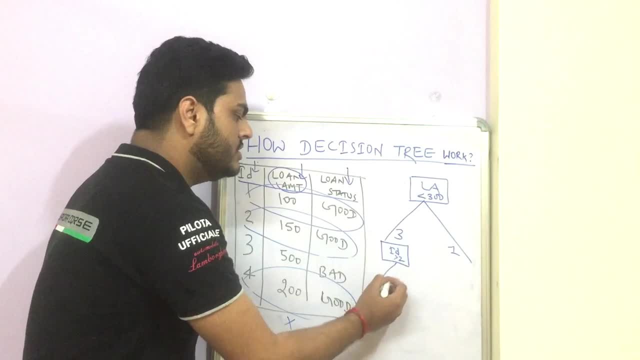 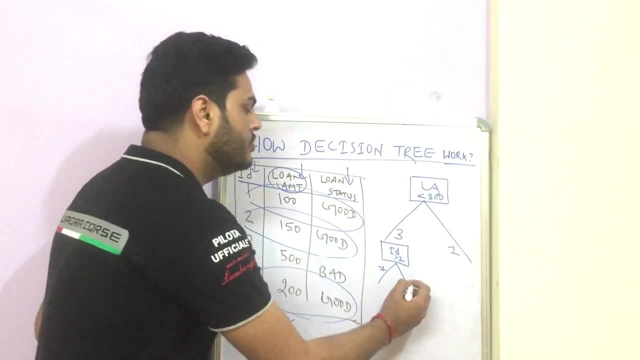 Okay. So here, when we say ID less than two and greater than two, then how many IDs are greater than two? only one ID four. So one comes this side and two record goes this side. Okay, These two records Okay. 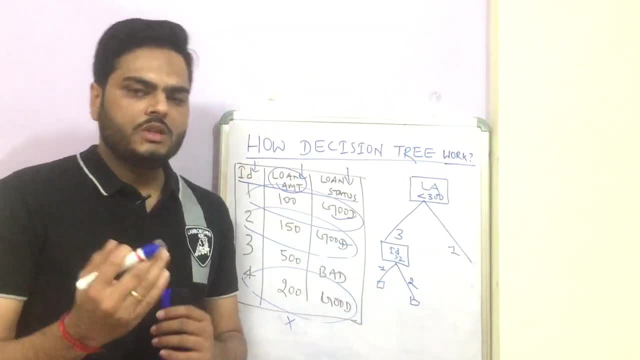 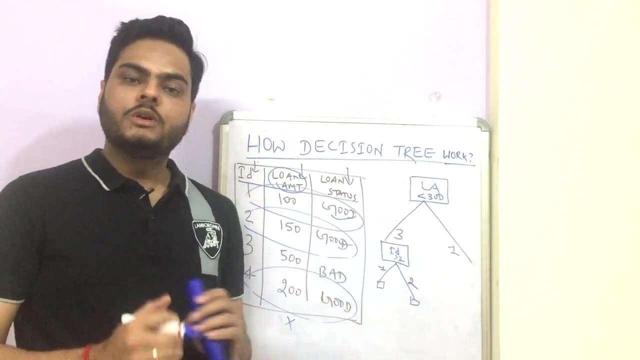 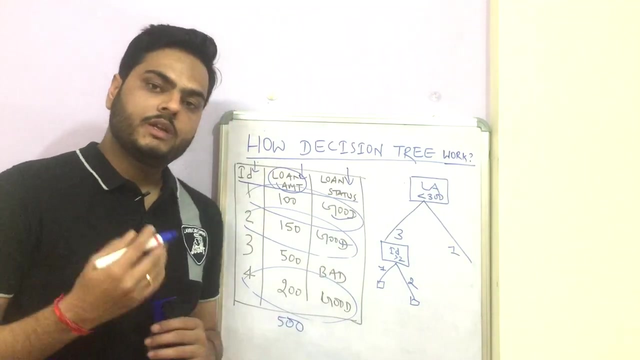 So this is how my tree is looking like Now. this tree is nothing but the model in this case, or the trend model in this case. Okay, So how the prediction will happen is tomorrow. I asked to this model: Hey, can you tell me? there is a loan amount of 500?. 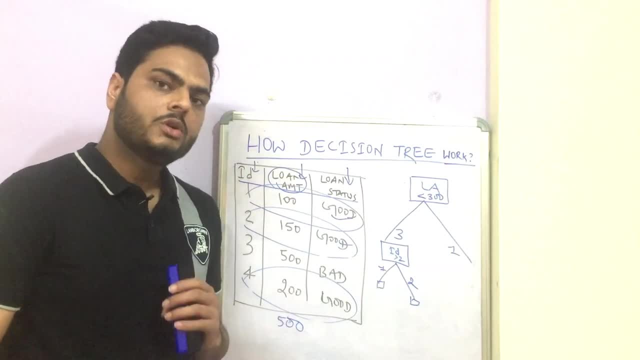 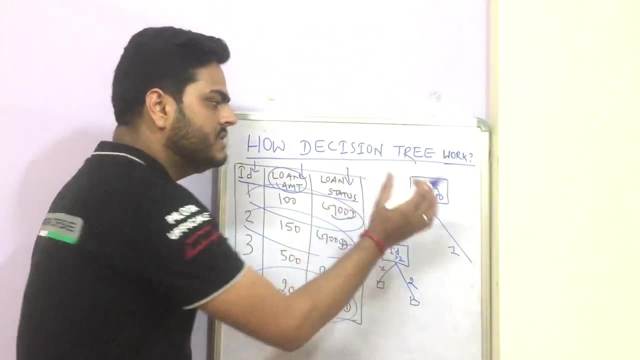 Can you tell me whether that loan amount will turn out to be a good loan or bad loan? decision tree will tell me: okay, look at, let me look at my tree and I'll tell you. So it will come here. It will check which side of the tree it will go in this side. 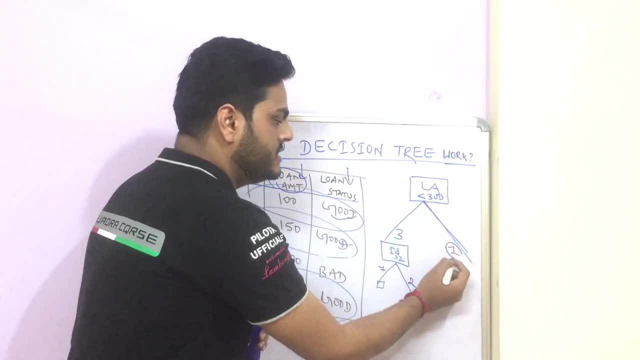 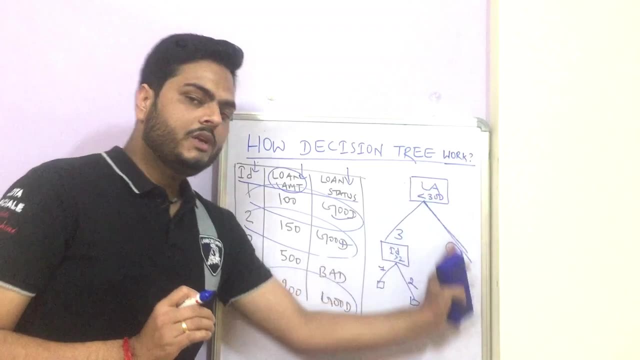 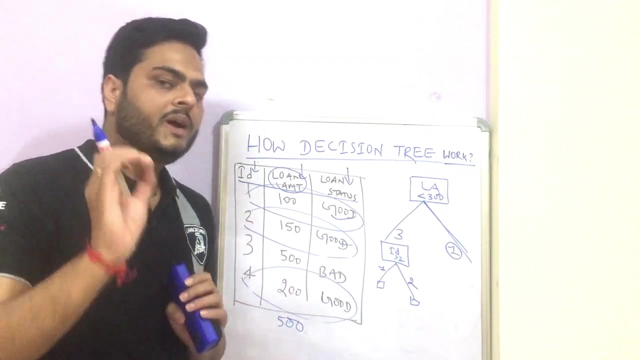 No, this side. it will go in. So this side. only one record is there. It will check the majority vote in that branch. I repeat it guys: Majority vote in that branch, which means in this branch whether there are more good loans or more bad loans. 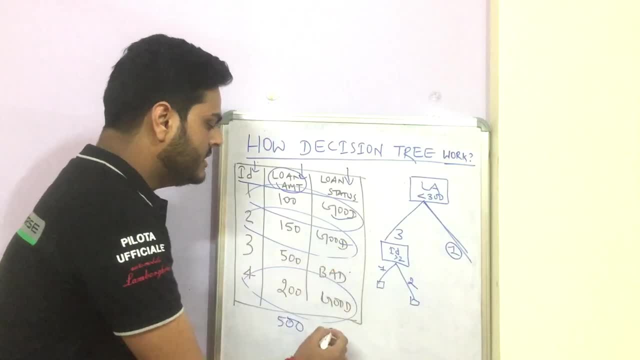 In this case, there is only one record which is bad. Hence the prediction happens to be bad. Okay, On the other hand, if I make it, let's say 200,. if I make it, let's say 200, and ID, I make it 2 and I ask to decision tree. 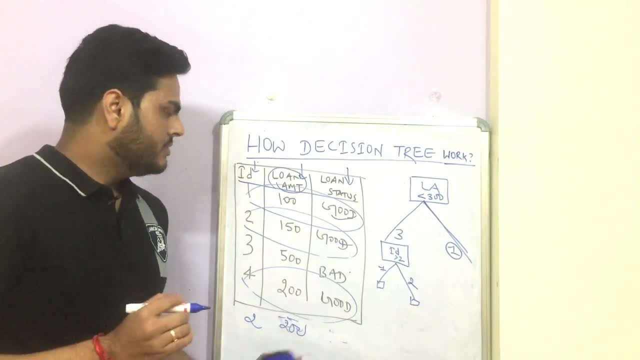 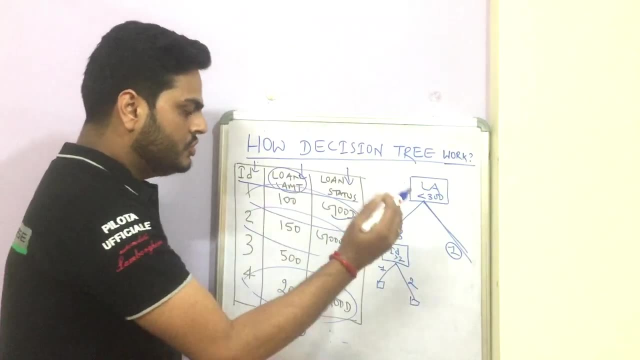 Can you tell me the prediction for this decision tree? will tell: Okay, So decision tree will come here, less than 200. come this side. check ID. ID is 2. each ID greater than 2.. No, which means go this side, this side. 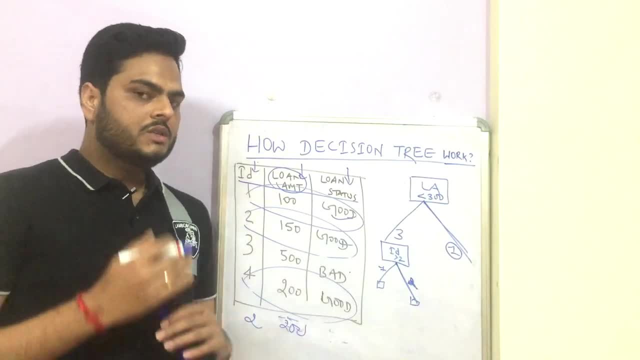 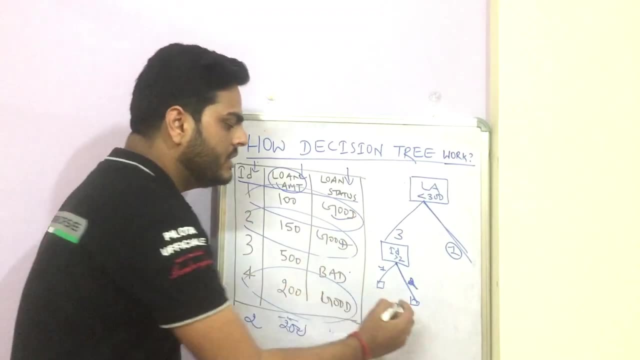 How many? 2?. So out of these two, What is the majority vote in this class? So if you see, both are falling in good category only, So there is good, only is the majority. Okay, so always. decision tree calculates the majority class. 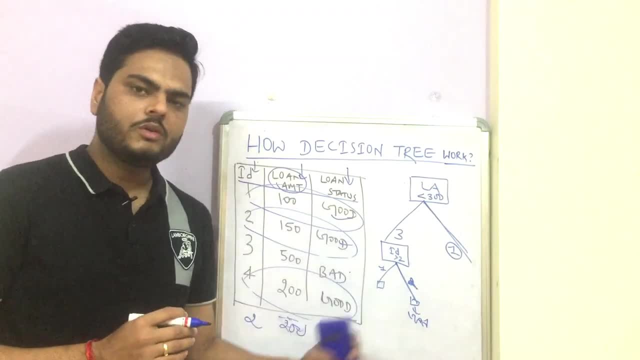 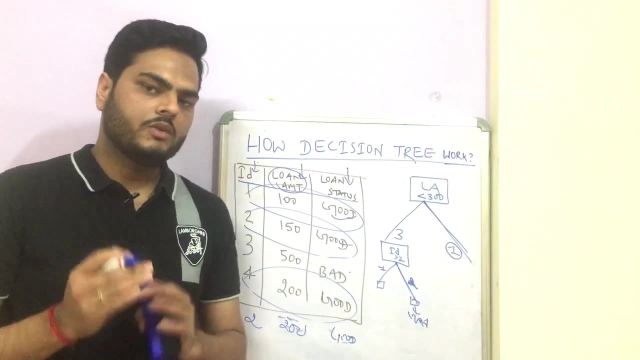 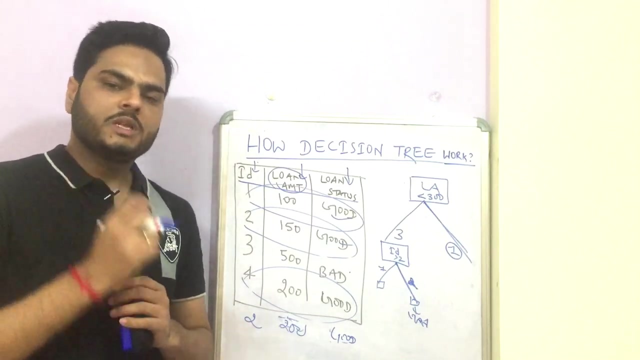 So here the prediction will be good. So this is how decision tree is trained internally and decision tree predicts the prediction at high level. Okay, in my next video I'll talk about those two important splitting criteria of decision tree, Which is little mathematical in nature but very important to understand one of the interview question as well. 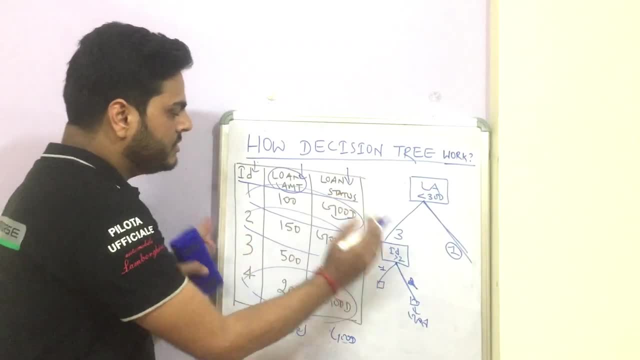 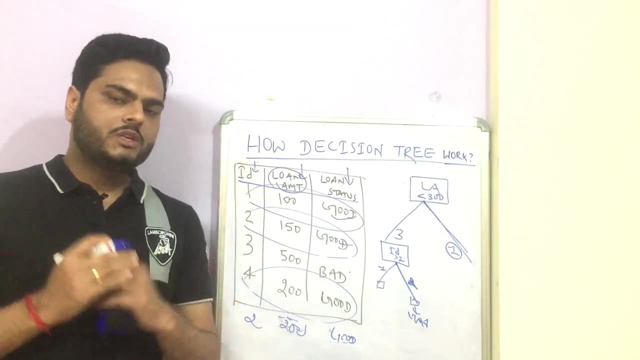 If you go for data science interview. So if you have any doubts on this topic, let me know through comments. Let me know through likes and comments. How did you like this video? I'll see you all in the next video. till then, take care.